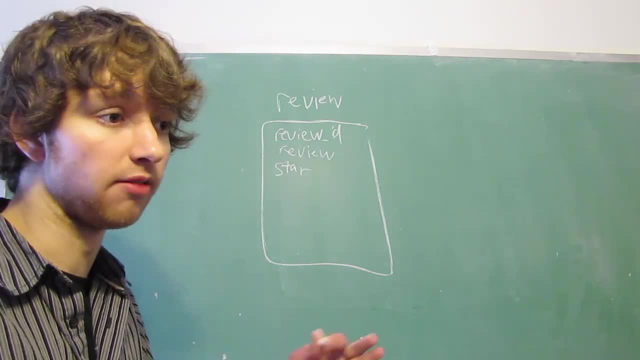 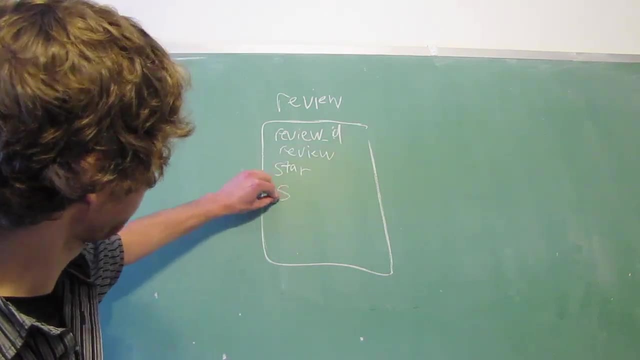 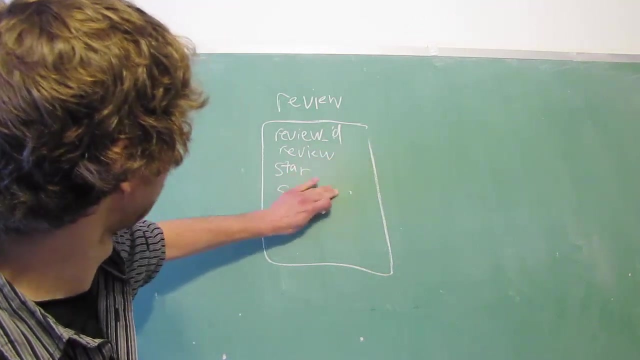 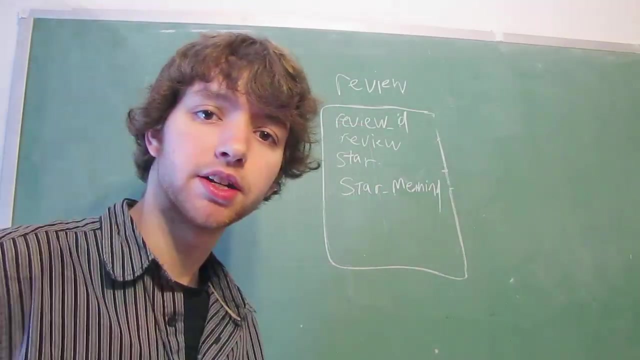 One being the worst, Five being awesome, And then four maybe being like really sort of okay, And then we might have something that has a star meaning, So that would be like sort of okay, Right, And finally we might have something like either a user or the poster. I'll just put. 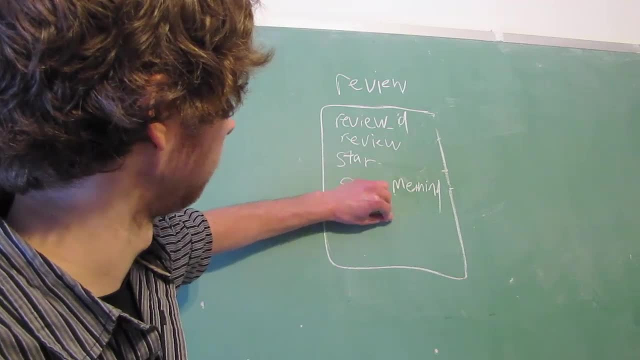 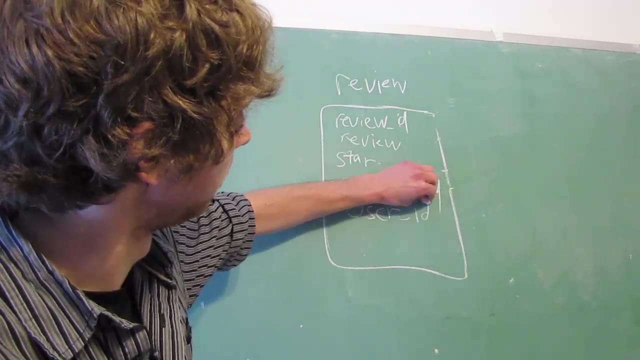 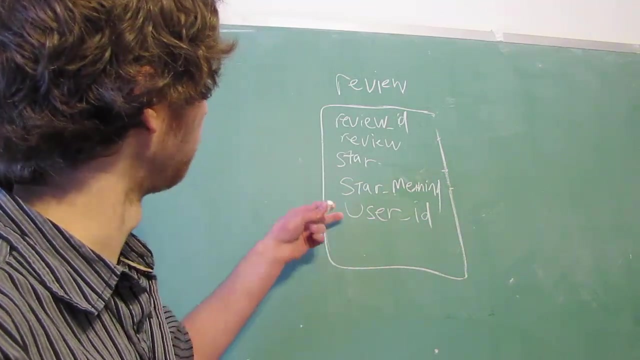 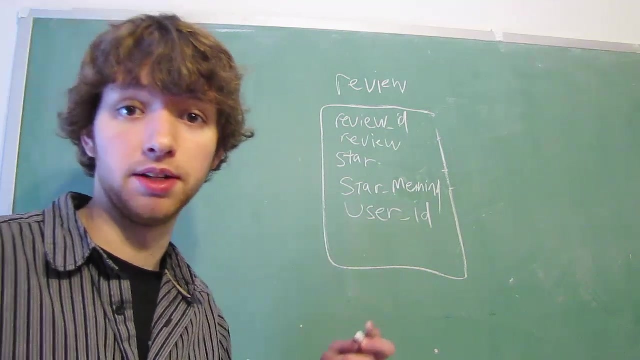 The user because likely you will have some kind of user account on this website where you can post comments. So this will likely be a user ID And it will be a foreign key to a user table. But we're not going to put that in here right now because that's unrelated to the actual point. So, foreign key, primary key. Now let's look at right here We have an issue. This is what's known as a transitive dependency, because the star meaning depends upon the star. 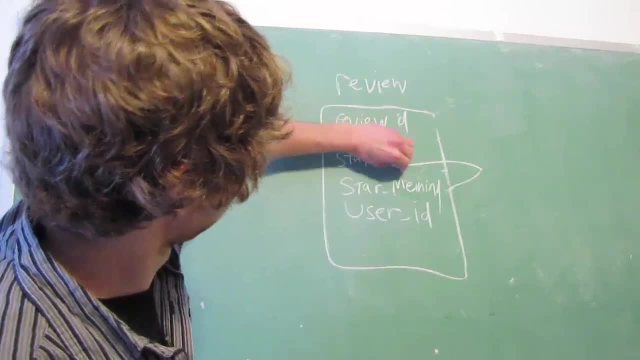 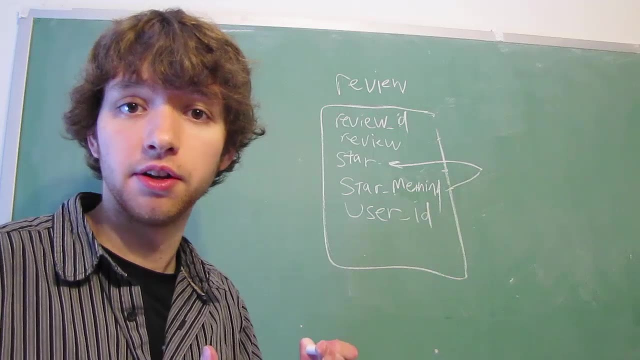 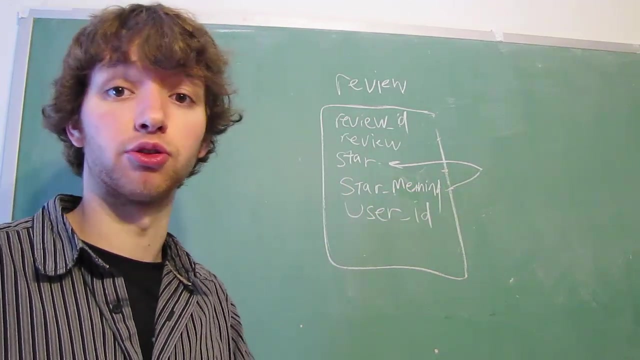 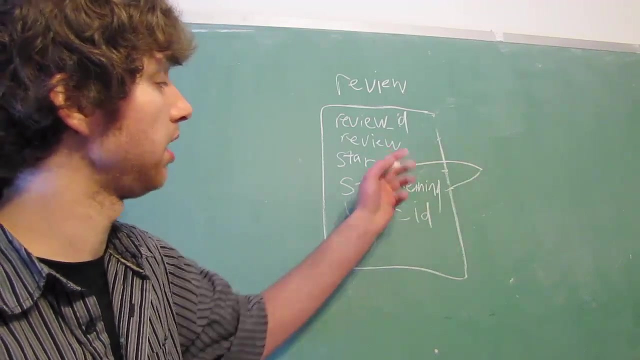 And a way you can kind of try to figure out. if it depends on it is okay. well, if we change the star, is the star meaning going to change? Well, if we take the star and we change it from a four to a three, it might go from. it might go from really super okay to really average. So the star meaning is going to change. So that's a dependency, But then the star actually depends upon the actual star. 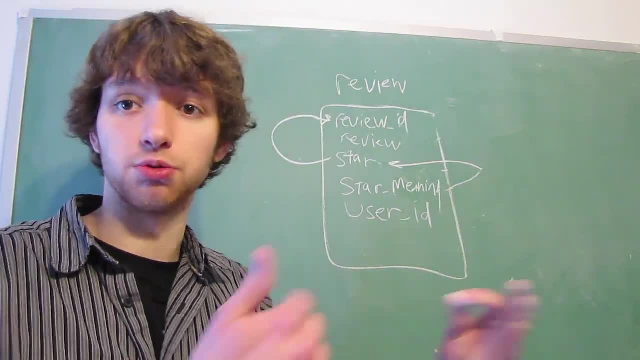 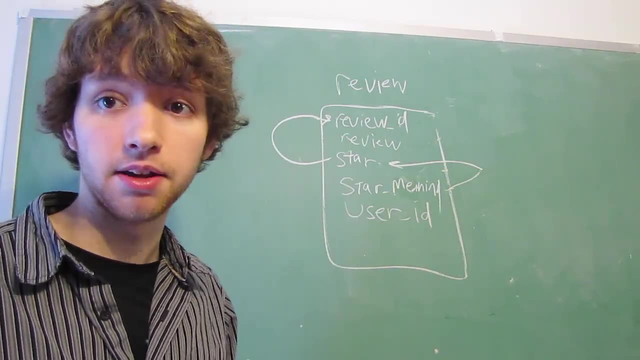 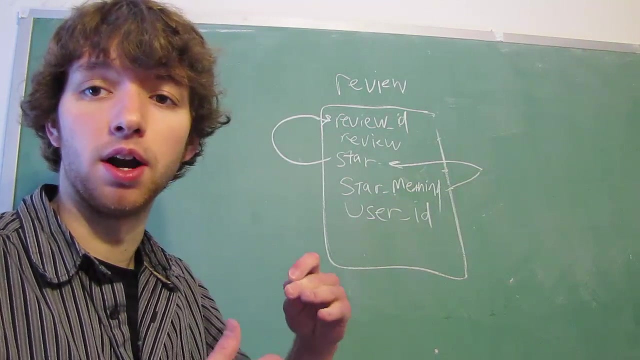 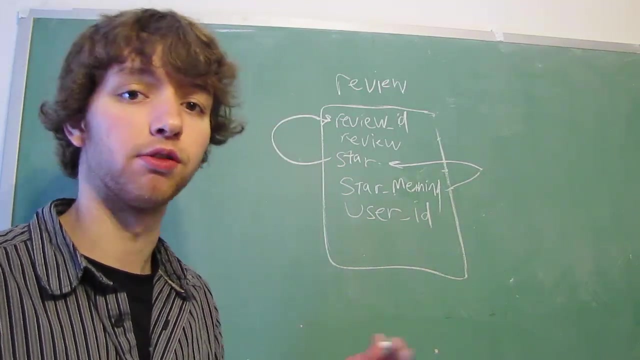 Review ID, because if you change the actual review, the star is able to change. So this is known as a transitive dependency, and it is bad. Now you can also have a multiple transitive dependency, which I don't even know what those are called, But that would be where a column depends upon a column which depends upon a column which depends upon a column which depends upon the actual primary key. It can go on forever, for as long as you want, But you don't want it because it's bad, which is why we're going to remove it. So to remove this, you take the columns that are causing a problem, you move them to a separate table and then you create a foreign key and replace of them which references the actual other column. So let's do this. So, since these columns right here are the ones causing the main problem, we take them, we put them in their own table. we have a star table. Within the star table we're going to have a star ID. 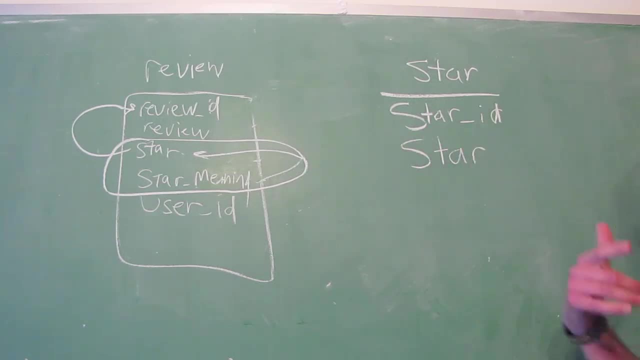 And then we're going to have the actual star, whether it be 1,, 2,, 3,, 4, or 5, or whatever kind of rating system you're using, And then we're going to have the star meaning. 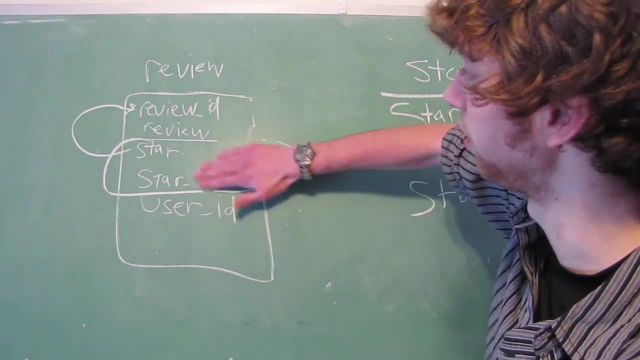 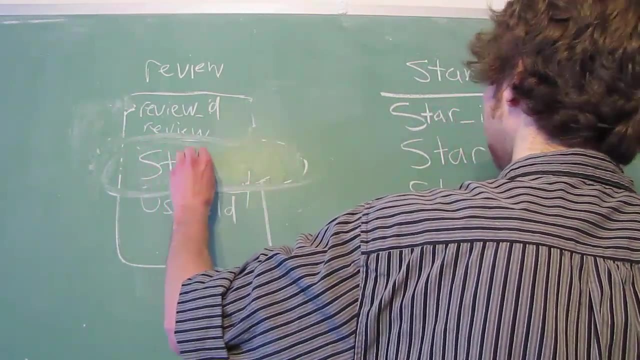 And then over here, we're going to replace these columns. Let me make this a little prettier And I just made it five times worse, But we're going to replace that with a star ID Which is going to reference This table over here. 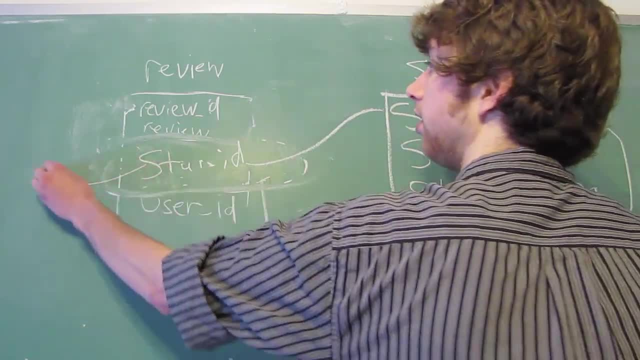 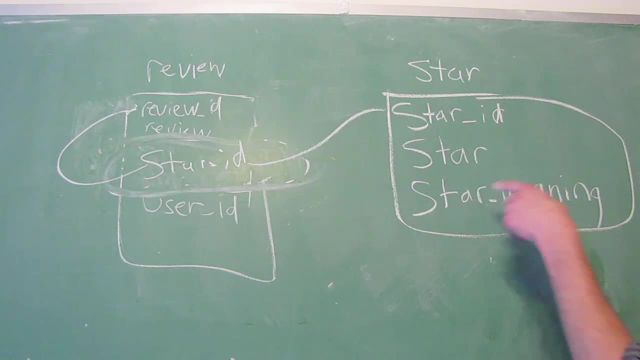 So now we don't have that problem because the only column over here is star ID. We don't have the star meaning, which was the real column that was causing the problem. Now over here we could have If we drew out this table we would have, you know. 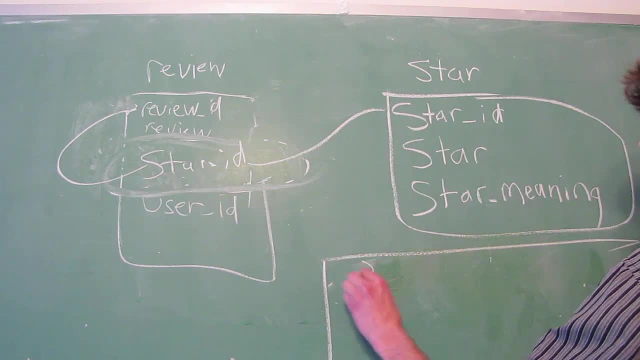 We could have a star ID of 3, and that star could be a 3 star rating and it could be meaning it could mean average. And that star could be a 3 star rating and it could be meaning it could mean average. 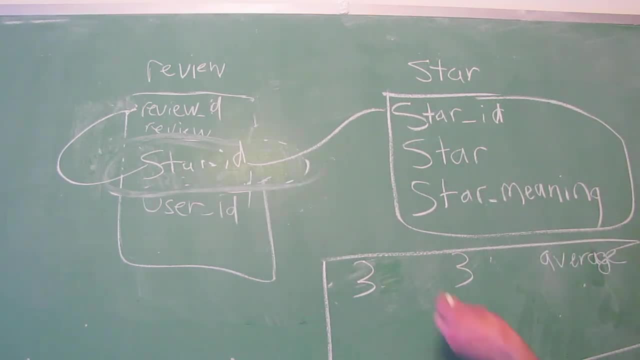 Now we're likely to only have five individual rows in this table, So it's kinda like a reference table. So over here we could have a star ID of 1,, 2,, 3,, 4, or 5.. 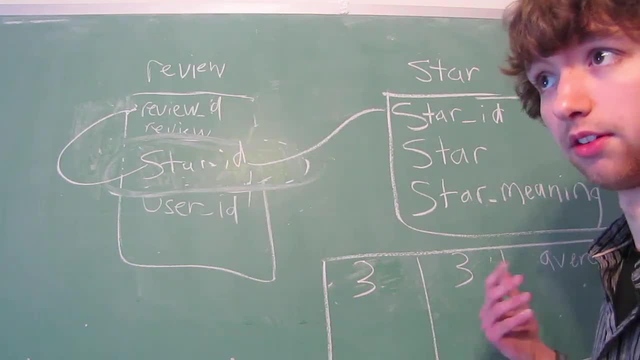 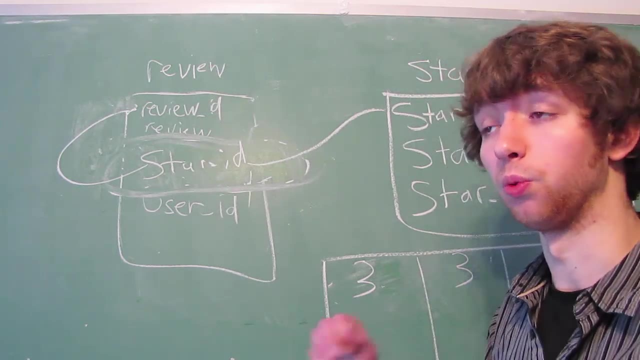 Or 0,, 1,, 2,, 3,, 4.. Or 5,, 6,, 7,, 8, 9.. It doesn't really matter what the ID is, because the ID is just a number used by the database and has no real world value. 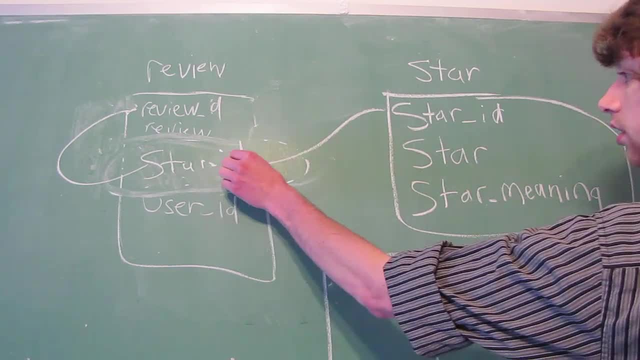 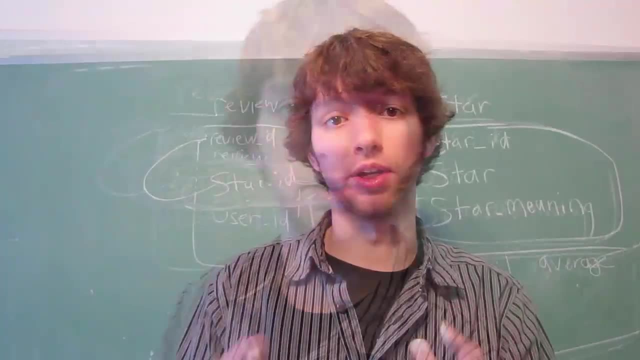 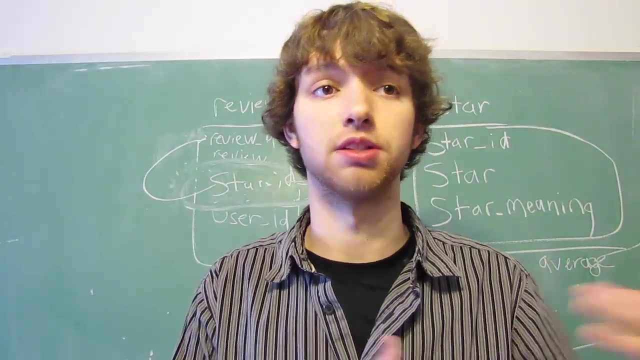 So we would have five rows in here and then we would reference them in the reviews table, So we could have: okay, this is too ugly, Let me just explain it. We could have one review with the star rating ID of five, which could correlate to a certain rating from this ratings table. 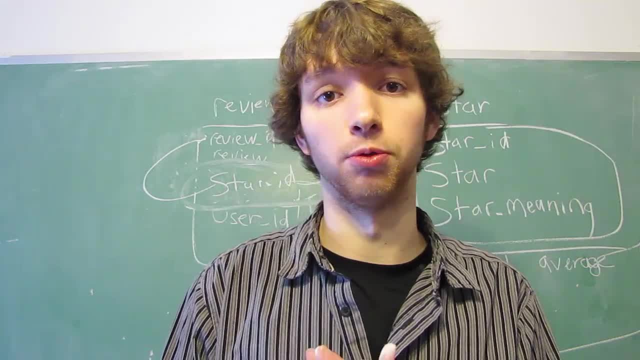 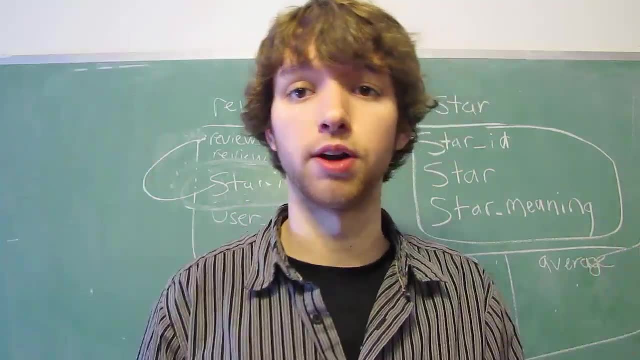 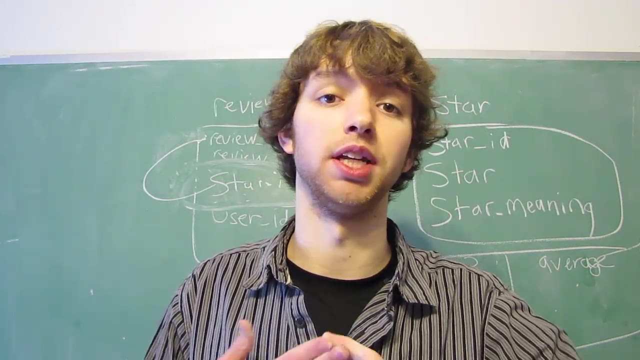 That's the main idea of the third normal form is to take those transitive dependencies, move them to a new table, create a forward key to reference that table. So in review: first normal form is making everything atomic. Second normal form is removing any partial dependencies. 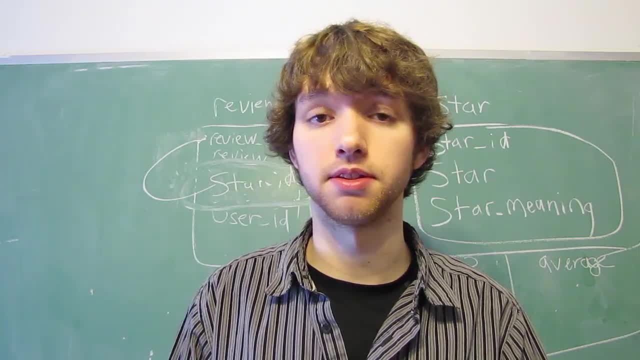 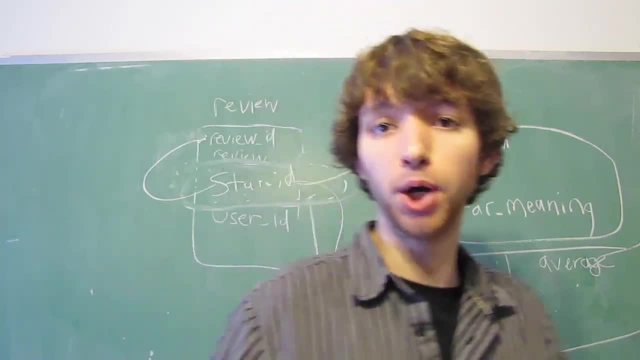 And then, third, normal form is removing any transitive dependencies. So thank you, guys for watching. I'll catch you in the next video, where we're going over something awesome Peace.